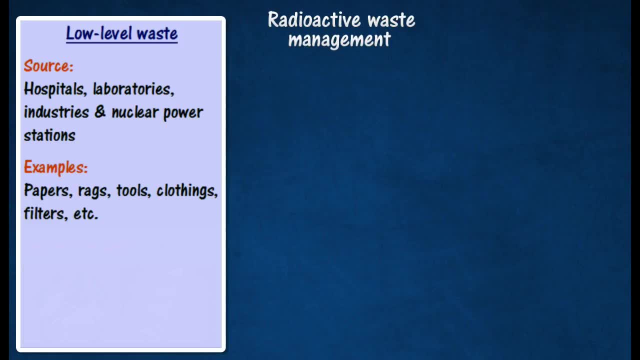 It comprises papers, rags, tools, clothings, filters and other object which contain small amount of mostly short-lived radioactivity. Such waste is not dangerous to handle but must be disposed of more carefully than normal garbage. It is usually buried in shallow landfill site. 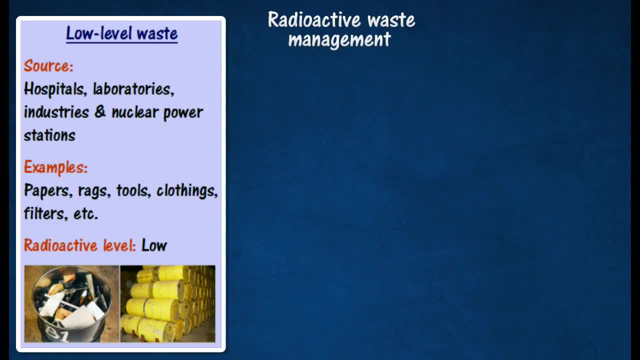 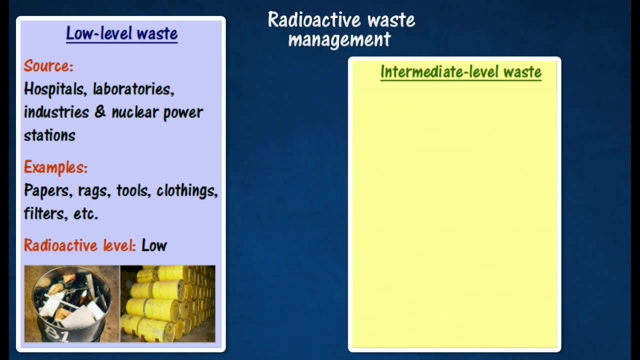 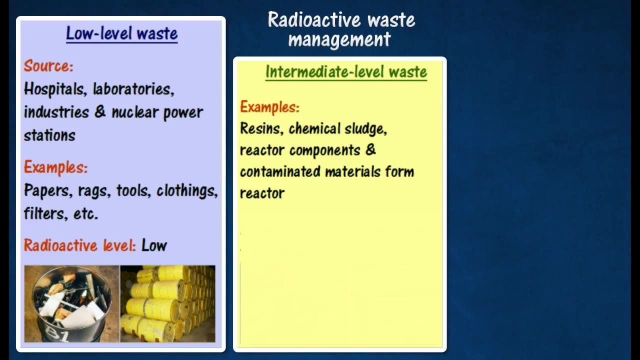 To reduce its volume, it is often compacted or incinerated in a closed container before disposal. Intermediate-level waste contains higher amounts of radioactivity and may require special shielding. It comprises resins, chemical sludge and reactor components, as well as contaminated materials form reactor decommissioning. 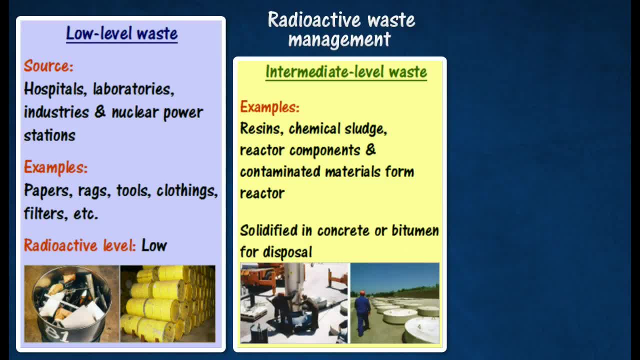 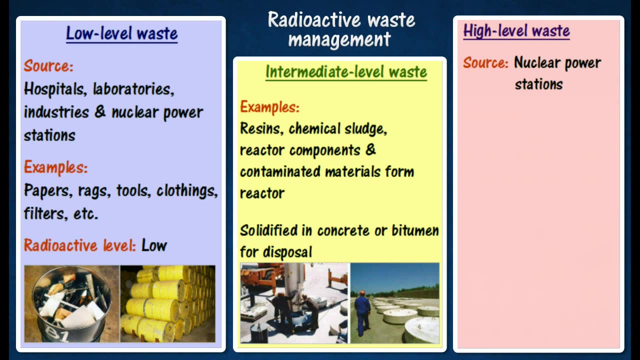 Such waste may be solidified in concrete encased containers and dumped in the ocean or buried deep underground. High-level waste accounts for over 65% of the total waste Total radioactivity produced in the process of nuclear electricity generation. Such waste is highly radioactive and it generates a considerable amount of heat, for example, fuel rods, liquid waste, highly radioactive fission products and some heavy elements. 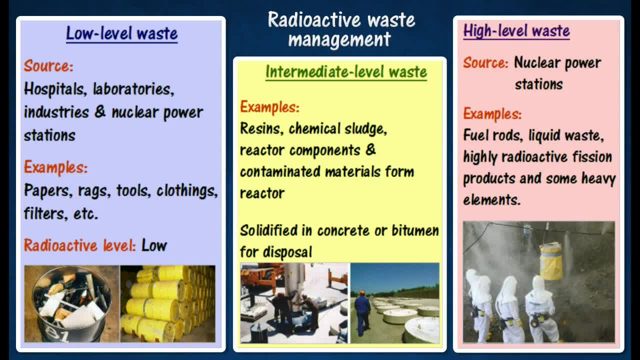